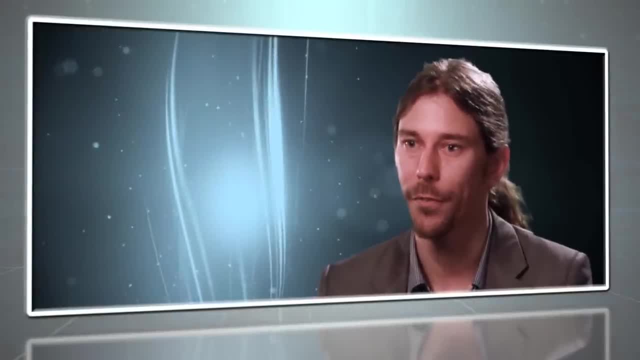 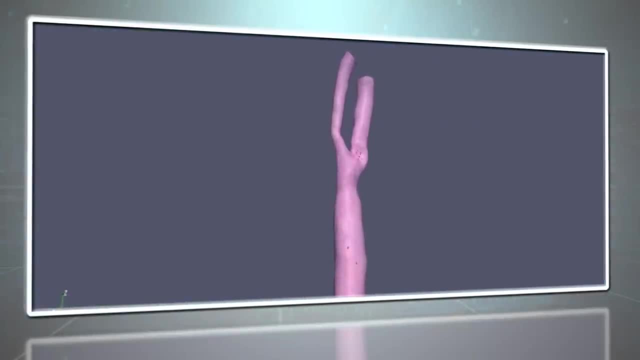 So one of the areas, one of the arterial structures that we've been focusing on, is the carotid. The carotid runs in the neck of the human body and it's an artery that splits in two, And this is a common area for plaque to build up, and these plaques can rupture or they can occlude the entire artery, which will cause strokes. 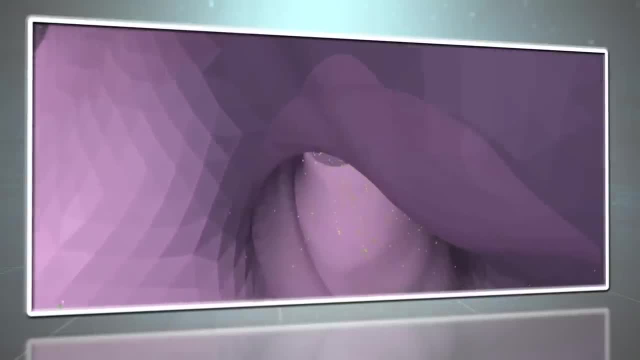 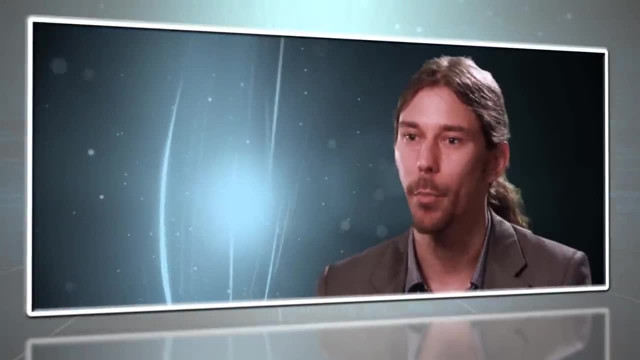 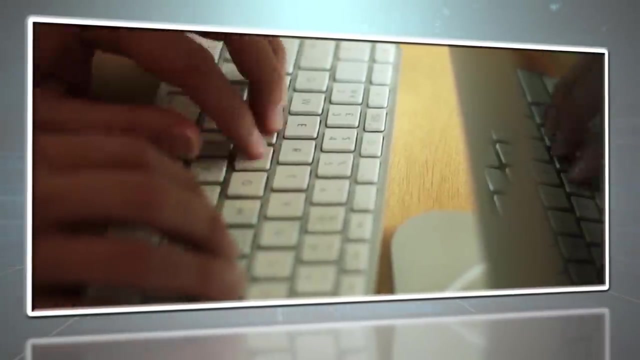 So what we are trying to do is to assess how the fluid dynamics and the mechanics and the interactions between the blood and the walls, how they link in with the biology and the progression of a plaque and the formation of a plaque, So we can use these studies to understand disease better and to come up with new, more advanced 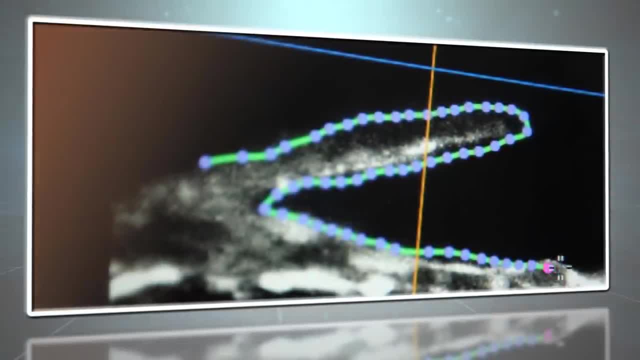 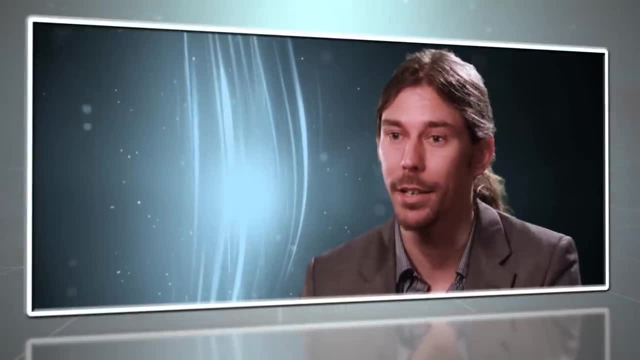 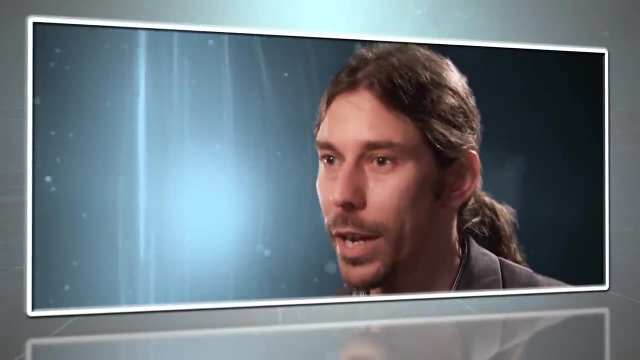 diagnostic criteria. A more recent example is a project that I'm doing in collaboration with Texas A&M and the lymphoedema clinic in Singleton Hospital. It focuses on the lymphatic system, which is essentially the system in your body that drains fluids from your tissues. 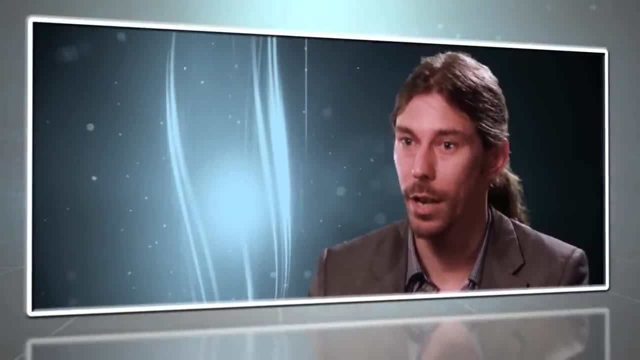 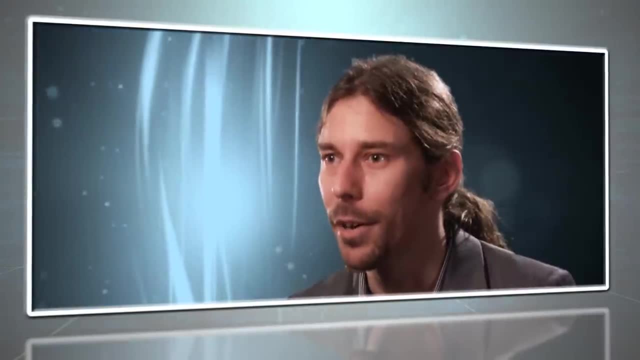 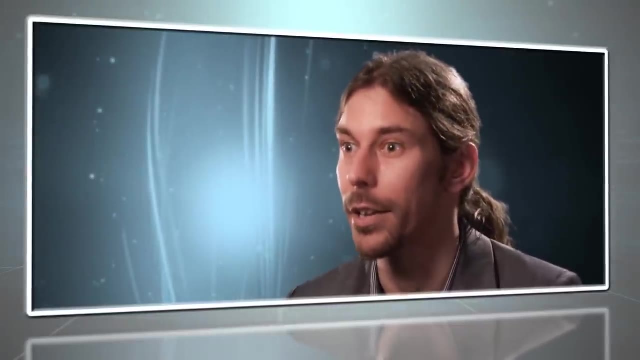 If it wouldn't drain these fluids, it would cause enlarged body parts, which is very uncomfortable and is a chronic disease. If you would have asked me a year ago anything about lymphatics, I wouldn't have known. But it was a professor in Texas who contacted me and said: 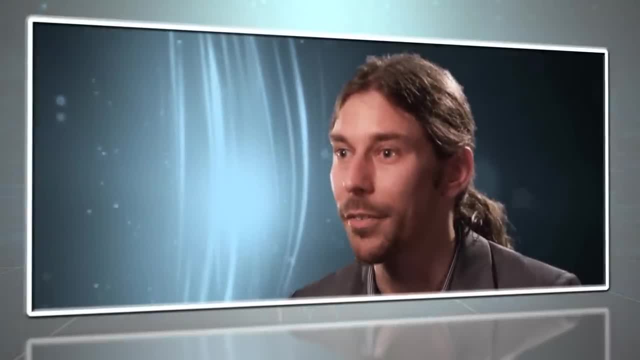 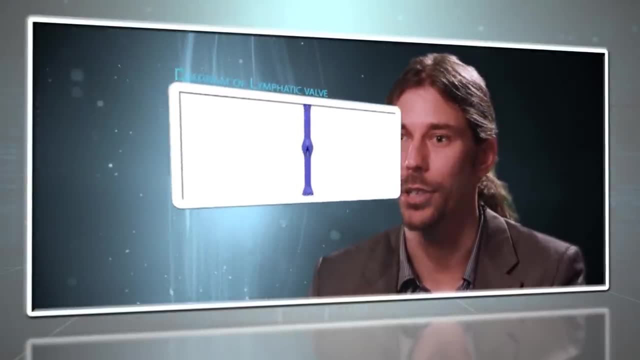 I know you work on heart valves. can you do something on lymphatic valves as well? So our research aims to study and analyze the contractility and the pumping function of the lymphatic vessels, And these vessels are as thin as a hair, with little valves in them. 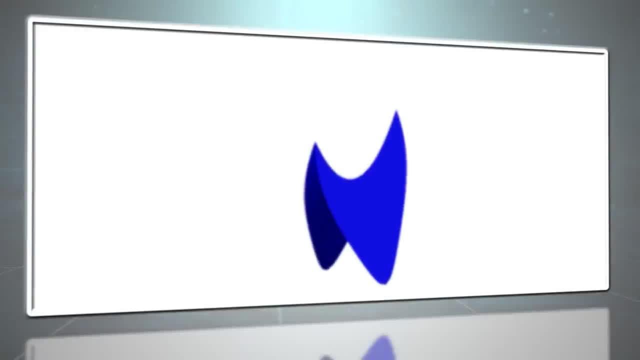 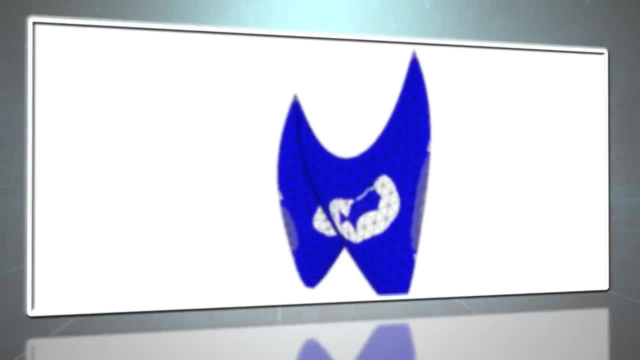 So if a valve closes, it causes pressures and stresses on the lymphatic system. So if a valve closes, it might causeWhich causes efflora on the leaflets and may cause that leaflets to fail. So once we understand the lymphatic pumping function better, 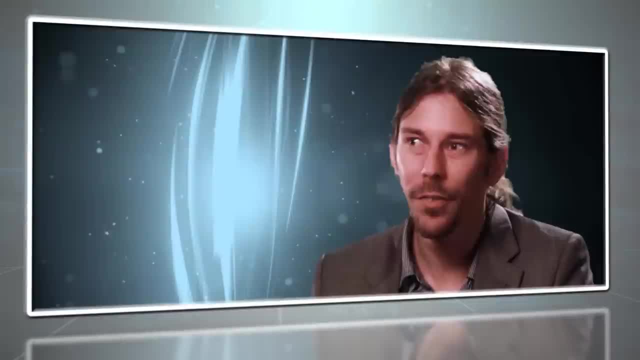 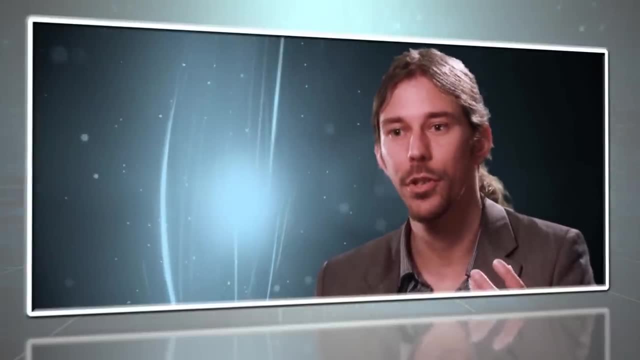 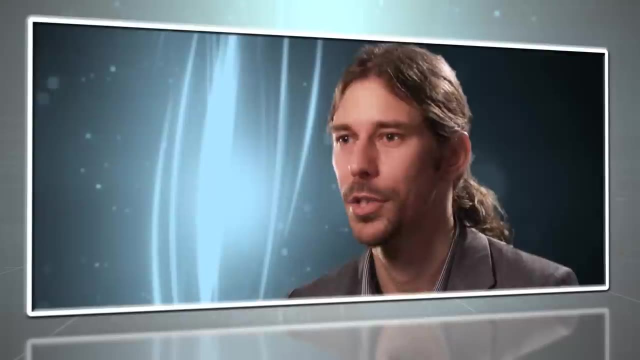 we can focus on optimizing treatment methods or develop possible new treatment methods. One of the directions I do want to take is to use my models- the mathematical and computational models- to translate them into the clinic, So actually use them in the clinic rather than sit behind my computer. 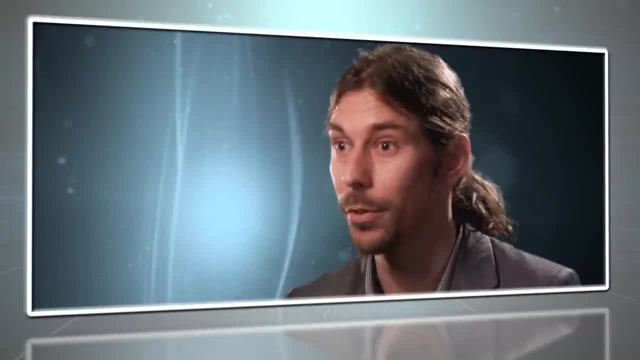 very big role in modern medicine and can help to improve clinical care.